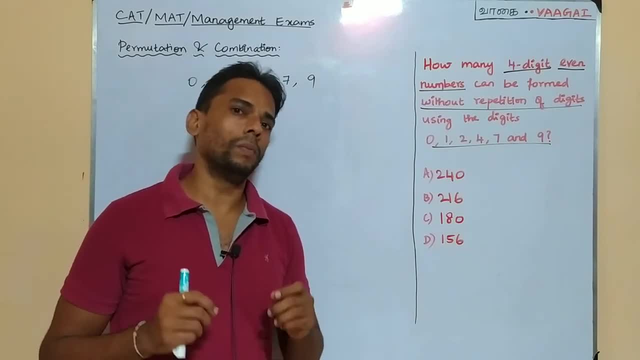 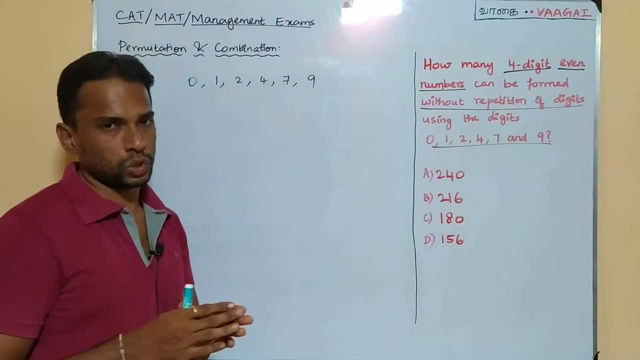 But this is going to be a little tricky. Okay, a little bit interesting question. We have to carefully work this question. that is really important And let us now see some good approach to solve this problem. Okay, let's work the question bite sized pieces. Okay, so we'll just. 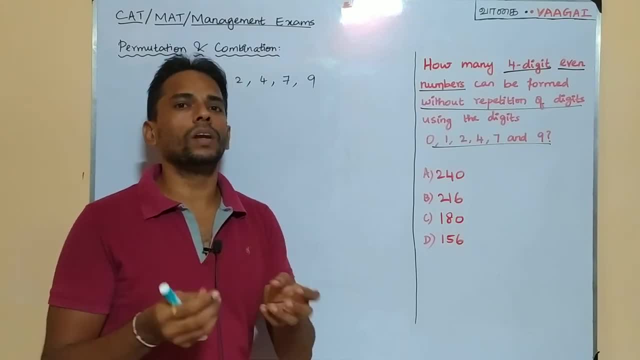 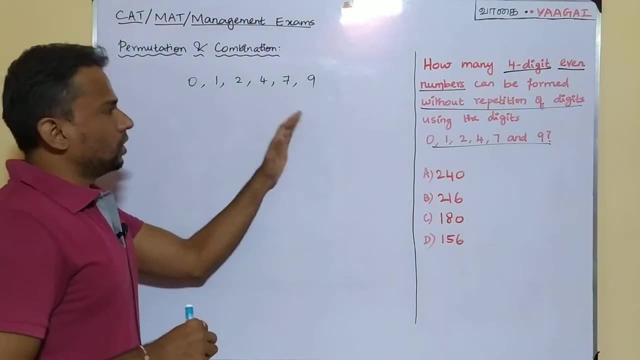 work the problem in piece by piece. Okay, only then it will give you a clear understanding. That's the reason, Okay, fine, Yeah, coming back to the problem, As we mentioned, there are six digits available here: 0,. 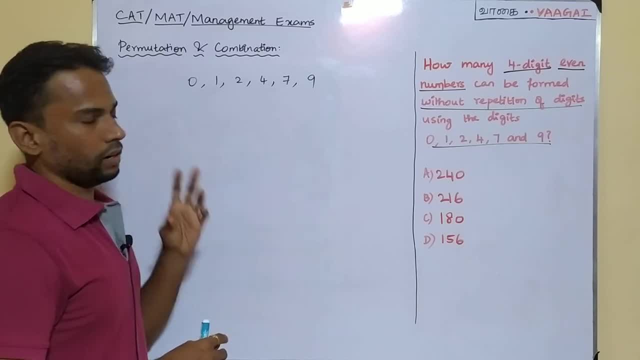 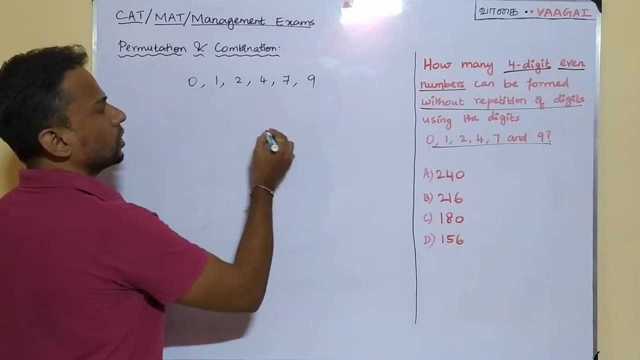 1,, 2,, 4,, 7, and 9.. And, using this, what type of number we have to form? we have to form a four digit number. Okay, so that means we should form a four digit number. So, dash, dash, dash, dash. 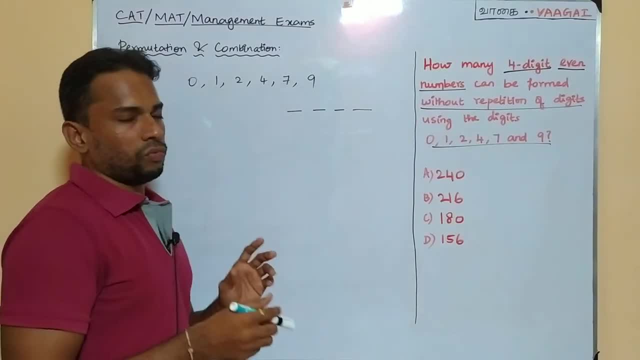 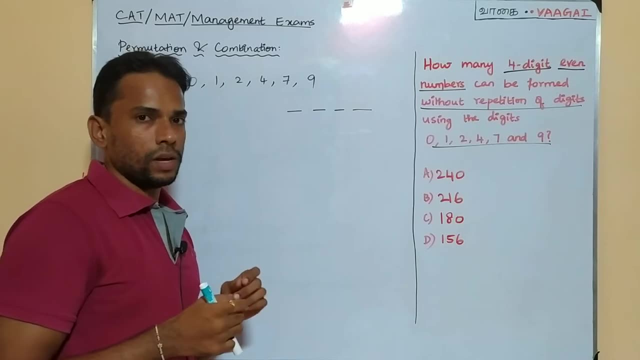 we have a four digit number, And that too, it is not just a four digit number, it is four digit even number. Okay, that is what the condition is given there in the question. So what do you mean by even number? the moment you see this condition- even number- what can you confirm? What can you? 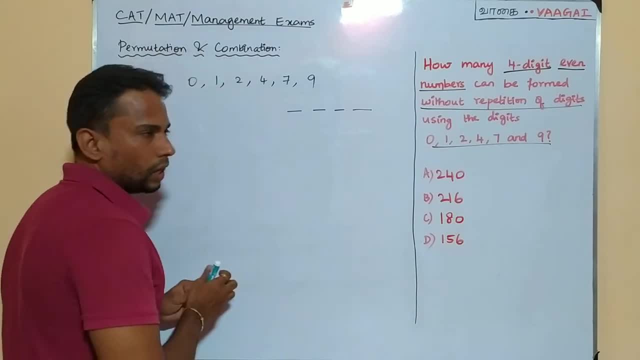 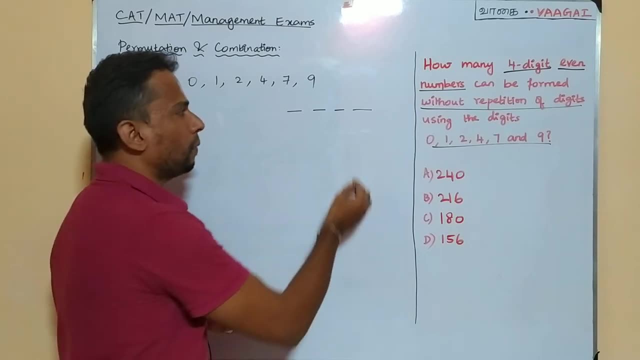 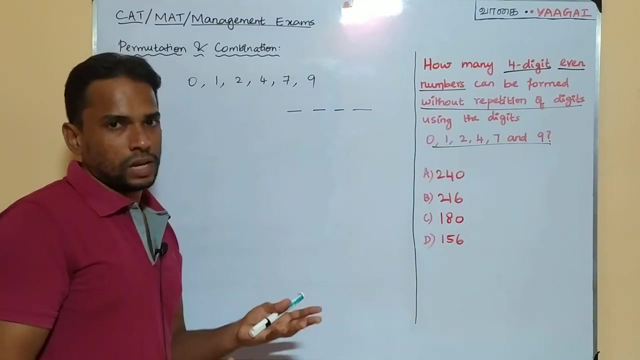 confirm about this number. We can confirm about the about the units place of our number. is it or not? Because for a number to be an even number, it is all decided by what digit we have at the units place. I mean the ones place. Okay, I mean the digit with which the number is ended. 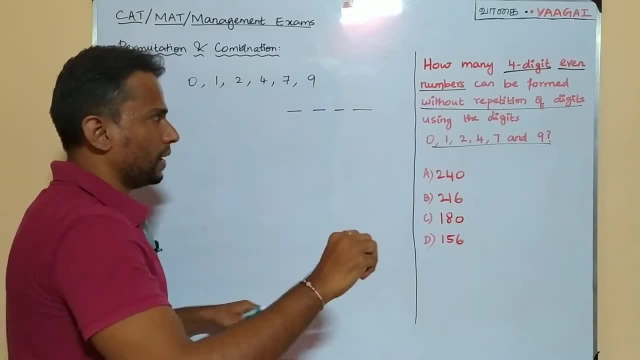 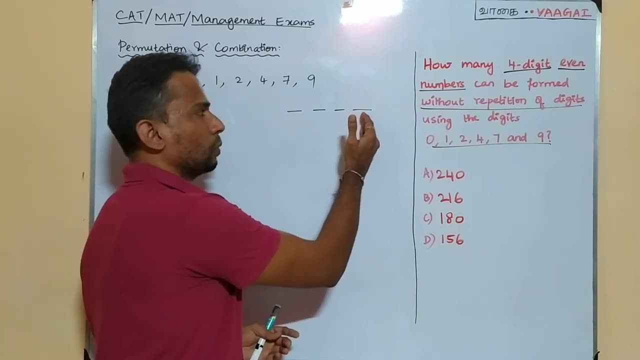 Okay, so this digit matters to be an even number. Okay, so that means, if you want to make this whole entire number to be an even number, this digit, what we fill here, this must be an even digit, is it or not? So that point we should be very sure at the first moment itself. Okay all. 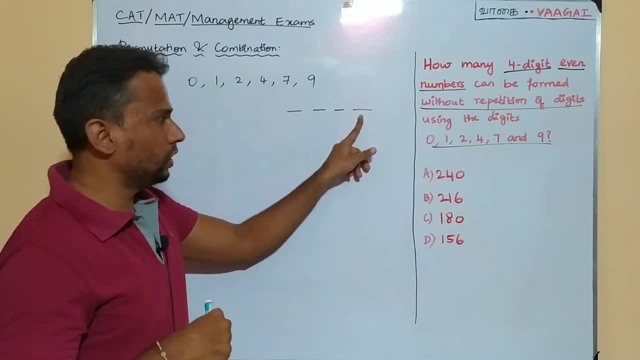 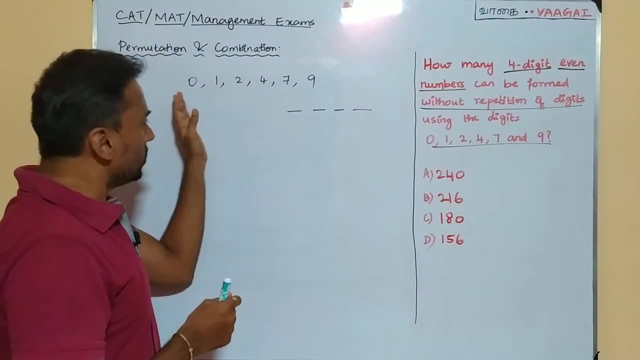 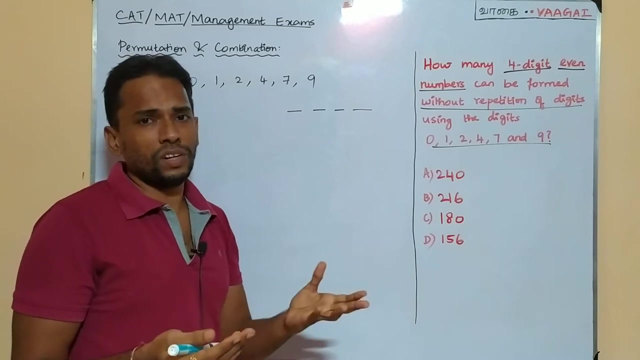 right, Yes, And now coming here, as we concluded, this should be an even digit, coming to our choices. Okay, now we have six digits here right Now. which among them, which among these digits, can be filled here that we have to think next? Okay, so what digits are all even digits, we know even. 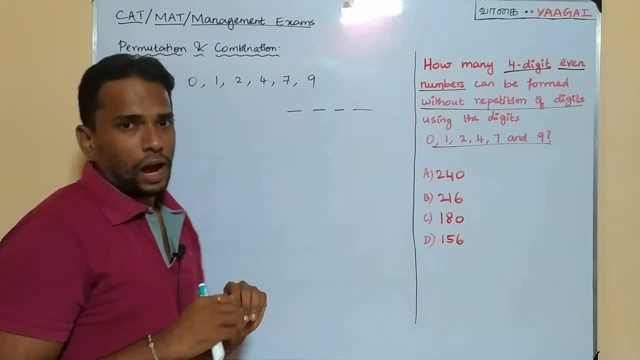 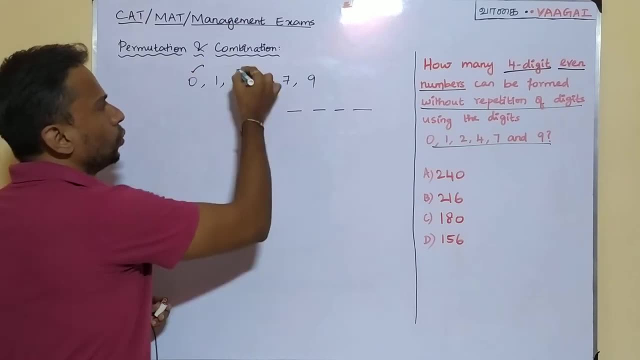 digits are 0,, 2,, 4,, 6 and 8.. Correct, Okay, And how many of them are available in our list that we have to see? So we have 0s here And 2 is another even digit. that is here, And 4 is an even digit. 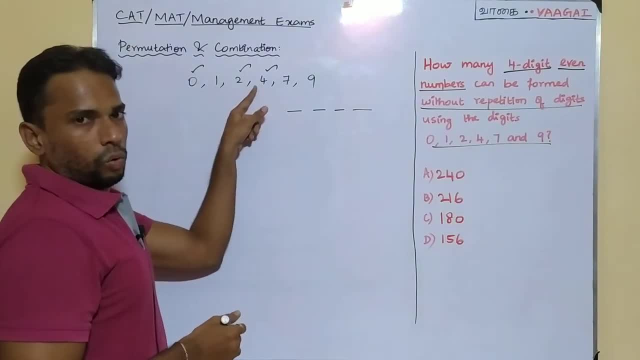 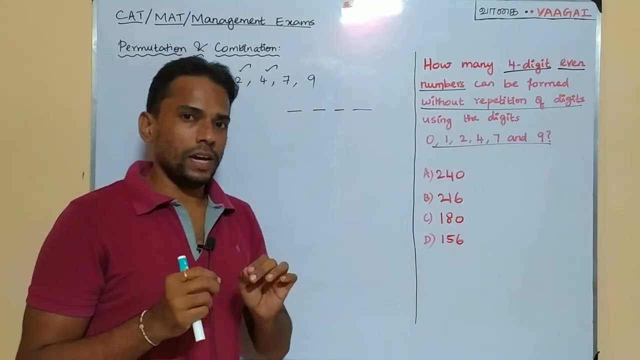 Correct. So that means either 0 or 2 or 4 should only come at this unit's place. That point we should be very clear. Okay, Now let us see how clearly we are going to work it out. Okay, fine, 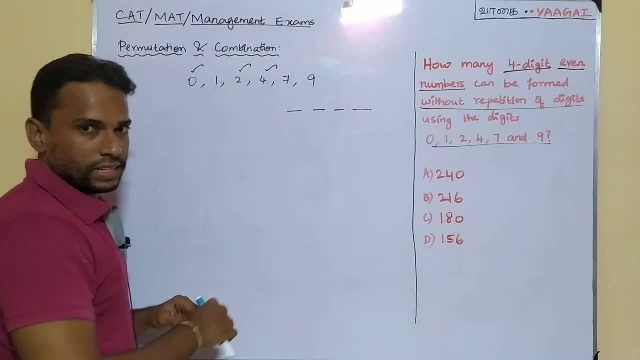 Yes, Let me just work the problem in three different cases. Okay, Why three different cases? You may ask the question For a clear understanding. I'm just trying to show in that possible way. Okay, fine, Yes, So let's work. Let's work the question in case by case. Okay, 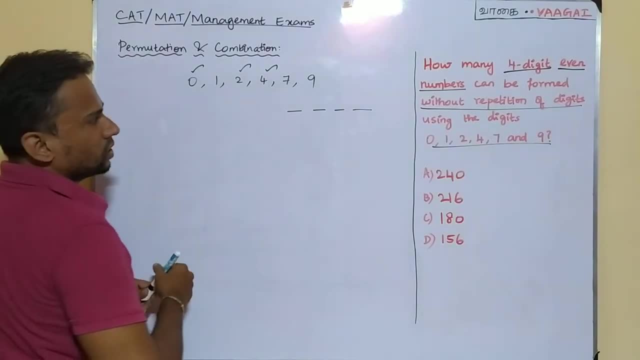 Case by case. we'll try to work the question, So we'll have it. First thing is here at the unit's place. since we have got three different digits with which it can end, right, So I'm going to make three different cases here. Okay, First case is ending with 0.. Ending with 0.. Okay So, 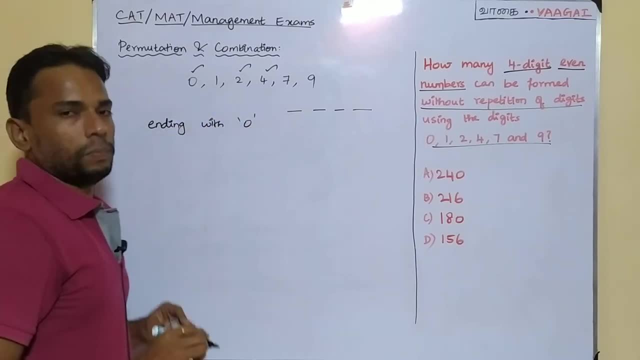 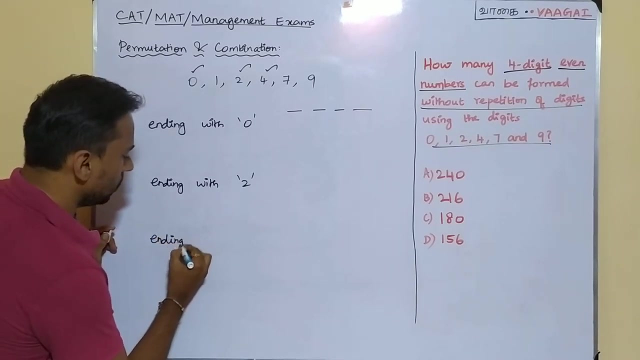 our four digit number is ending with a 0. Then what will happen? Fine, Okay. And next, what if our four digit number is ending with ending with what is the next even digit? Next even digit is 2, right Ending with 2.. Now what happens? And last case is ending with ending with what is. 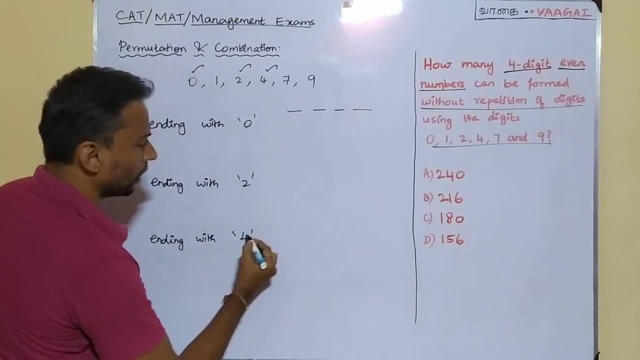 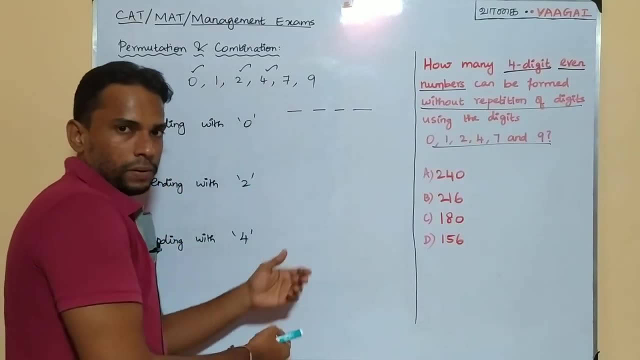 other, even digit, It is 4 here. Okay, Ending with 4.. Now what happens? Okay, So we will work out each of these cases separately and then we will finally add everything. Okay, Why? Because our answer should be either of any any one of these cases. only right: Either this or this or this. 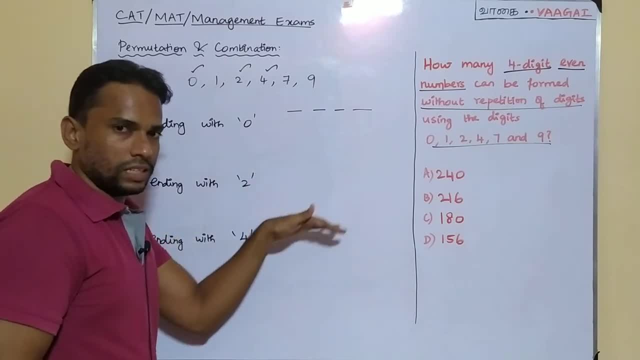 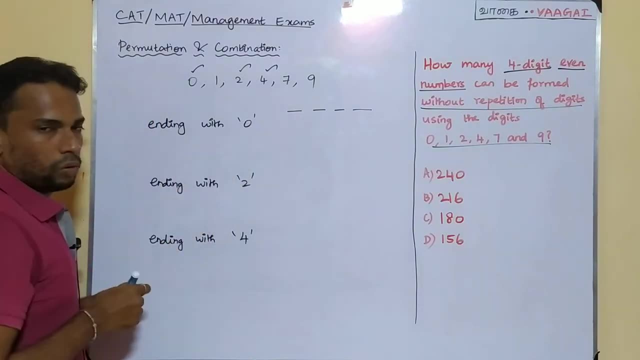 So, finally, we will add all these answers, Okay, All these cases, values, and that will give you the final answer. Okay, Is it or not? So let's work the the first case ending with a 0.. Okay, So that means dash, dash, dash, dash, This last. 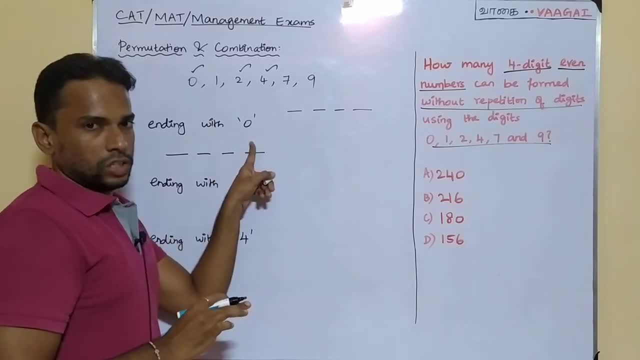 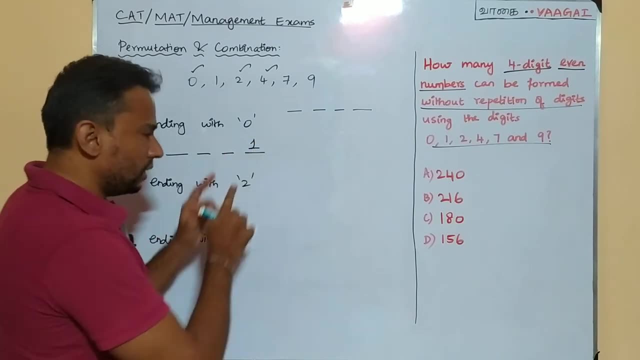 slot is filled by 0.. Okay, Now let us not touch this. Okay, This is filled by 0.. So that means this is filled with that one possible way. Okay, Why I am writing 1? there is that is fixed That. 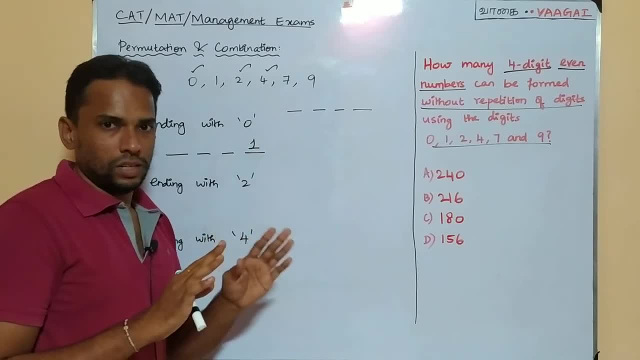 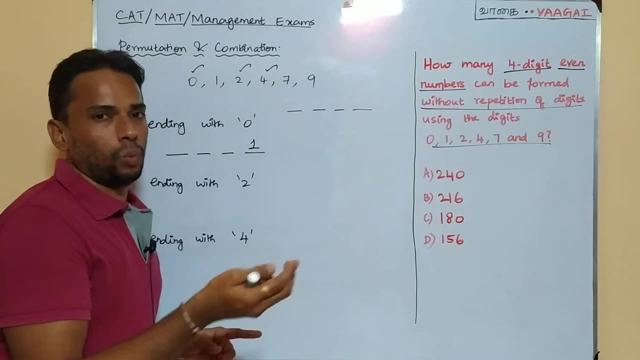 is only filled with 0. There are no other digits possibility Coming there. That is the reason I am filling this 1 here. Remember: this 1 doesn't stand for the digit 1.. Okay, It stands for. the only digit that comes here is the digit 0.. Okay To represent. 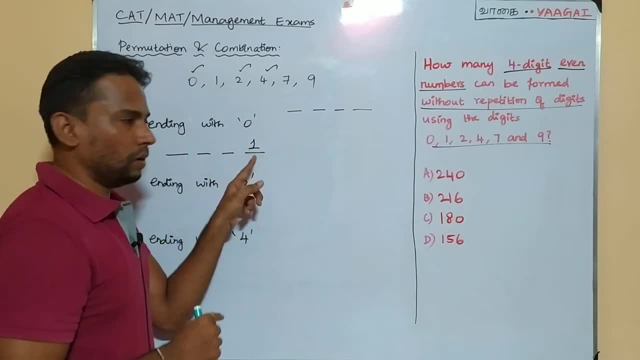 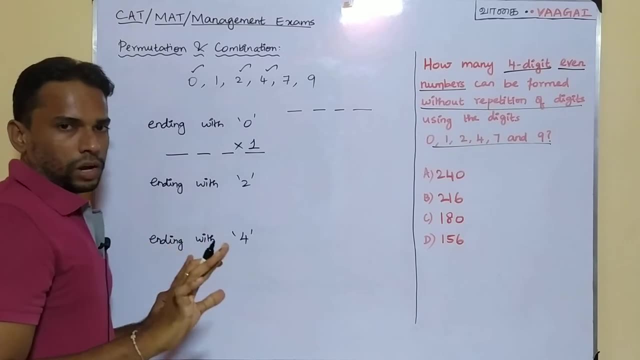 that only there is only one digit coming here. There is only one possible way. I am filling that 1 here. Okay, All right. Yes, So that means we have filled this digit with the digit 0.. Okay, All right, Yes, That is done Now. now remember there are other 3 slots there. Now these slots. 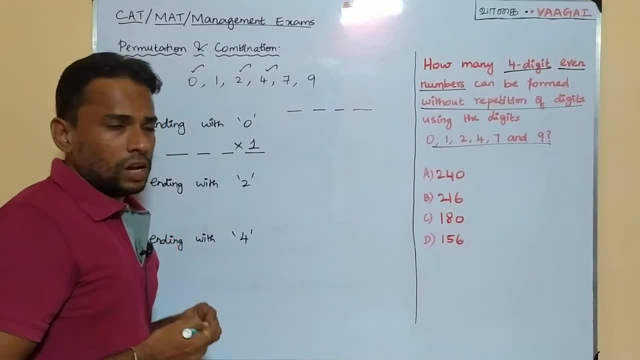 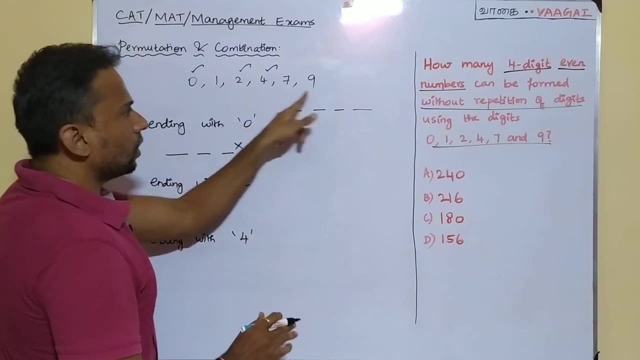 are filled with any conditions. Do you have any other conditions here? Now? what are the other digits left? We have the other digits left, are? we have filled 0 here? Okay, So the problem is over. What are the other available digits here? Here we have the digits. Let me write here: Okay, 1,. 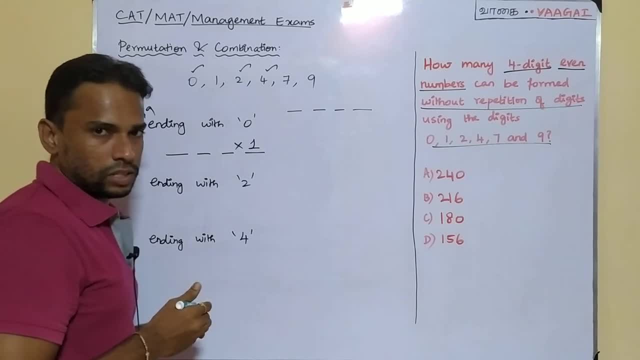 2,, 4,, 7 and 9.. These are the other available digits. Yes, Okay, Now we are going to fill these 3 slots using these 5 digits. Is the point clear Hereafter? do you think there? 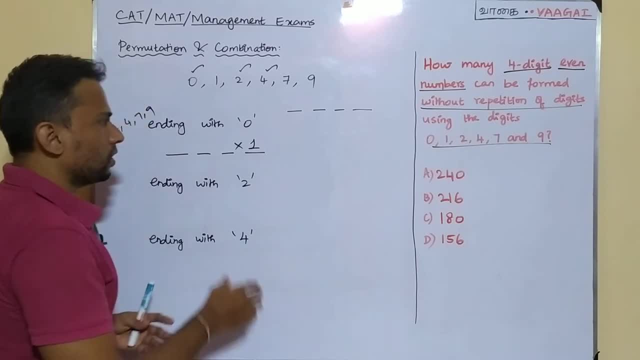 are any other conditions? are there? No other conditions are there? Okay, Now we are going to fill these other conditions, Right? Why? Because we have filled the 0 here. Now remaining 5 digits are here. I can fill these 3 slots with any of these 5 digits. I mean any 3 of. 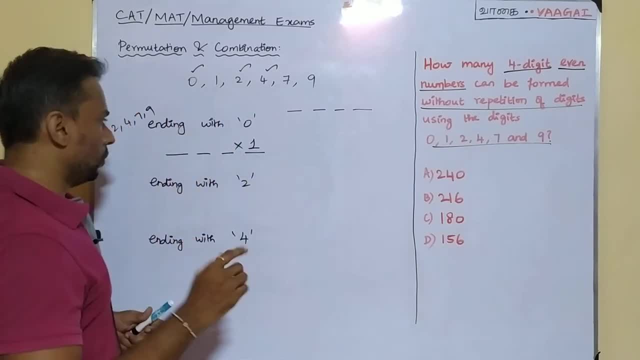 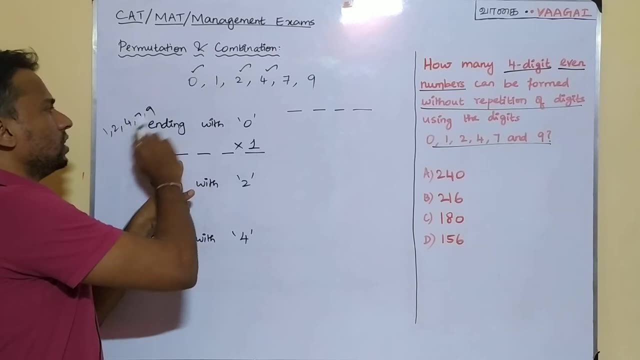 the other 5 available digits. That is what I mean. Okay, Now, in that case, now come here. This first slot can be filled in how many ways? This can be filled with any one of these 5 digits, Is it or not? So that means this first slot. we have got 5 ways, Remember. 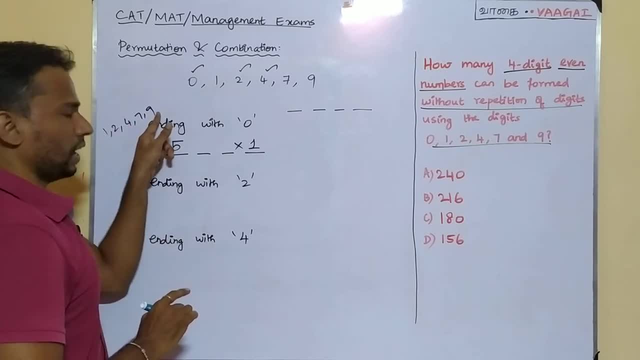 there are 5 ways, because I have 1 or 2 or 4 or 7 or 9.. Any one of these 5 ways I can fill 5 digits can come here. So I have got 5 ways in which I can fill this slot multiplied. 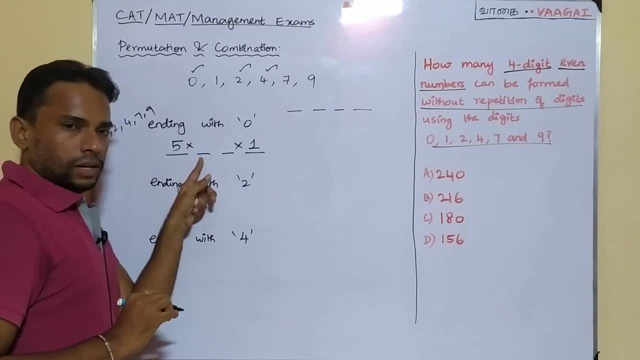 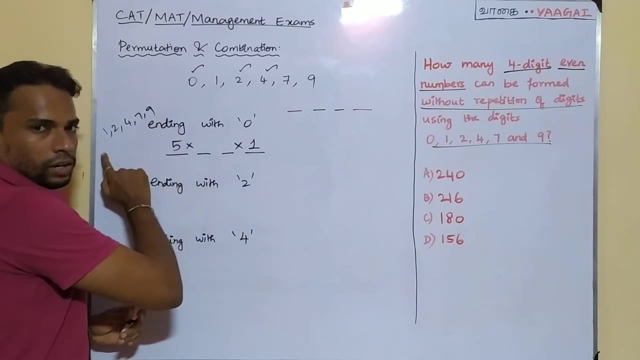 by Now. coming to the second slot Here. when I come here now, how many ways will be there? There will be only 4 ways available. Why? Because any one of them? Okay, Already, any one of them would have filled the first one. Okay, Fine, Yes, Now, when you come here, 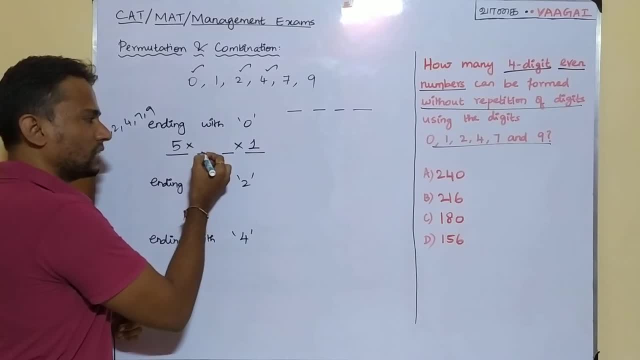 there will be only 4 choices, Correct, Okay, So that means when you come for the second slot, there are 4 ways to fill the second slot. Again, when you come to this third slot, one more is reduced Out of 5.. 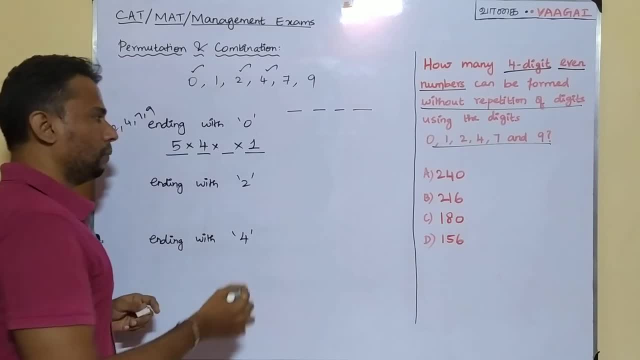 2 are filled, So there will be only remaining 3 digits available. So this can be filled in 3 different ways. So that means what is the total number of ways here? Just multiply everything 5 into 4, into 3, into 1.. So that will give you the answer as 60. Right So? 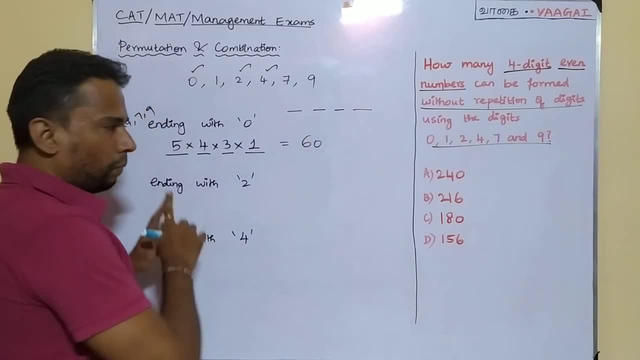 that means there are 60 ways with which you can form a 4 digit number which is ending with 0. Clear, Is the point clear? Okay, Fine, Alright. Now coming to the second case here. Second case says ending with the digit 2.. Okay, So this time we are going to fill our 4 slots in such a way that 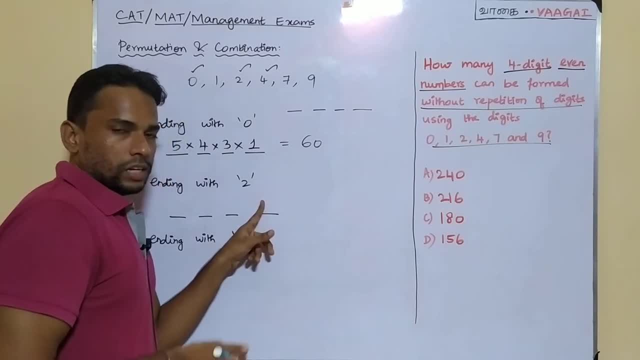 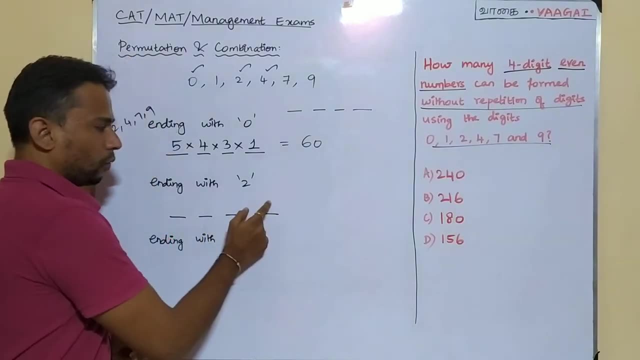 now, this time, this ending digit, unit digit, is now filled with the digit 2.. The digit 2. This is the meaning. Okay, Alright, So now I am going to fill this digit with the digit 2.. Again. 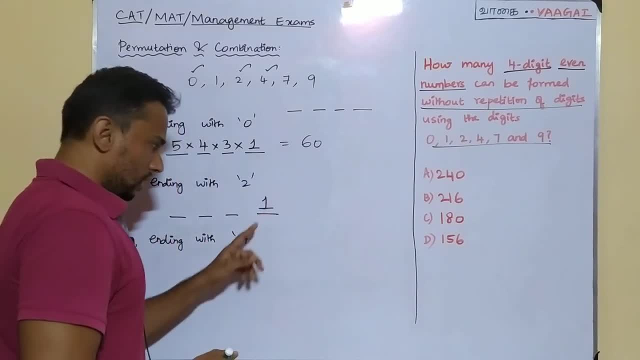 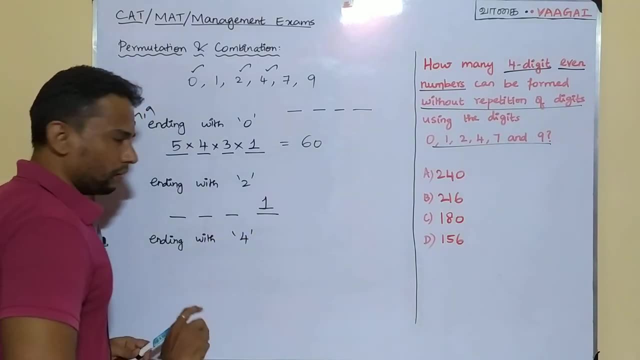 to represent that I am going to put 1 here, stating that this is filled with the digit 2.. There is only one possible way, Okay, To represent that I have filled this. Okay, Now think again. think here When you come to fill this. 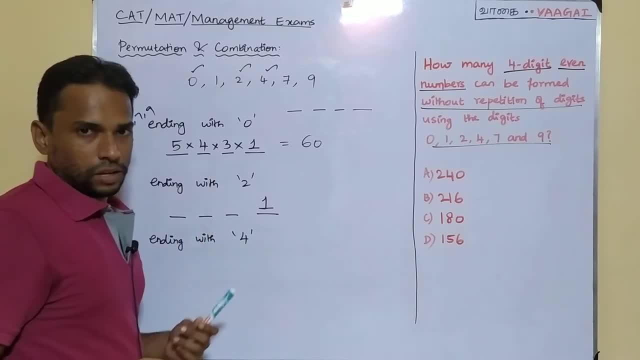 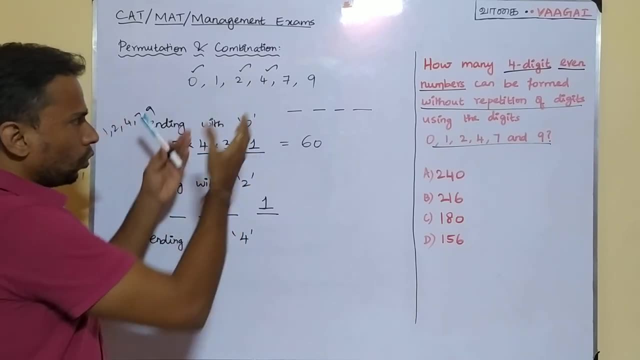 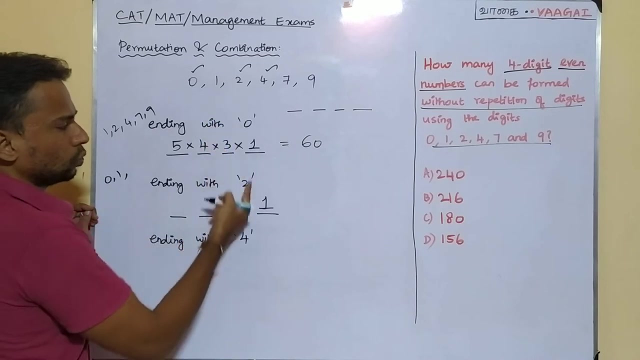 digit with 2,. now what are the other remaining digits here? What are the other digits which are left over now? So other digits are here we have. we have filled with 2.. Correct, Now note down the other remaining digits. So we will be now left with 0, then 1. Leave this 2.. 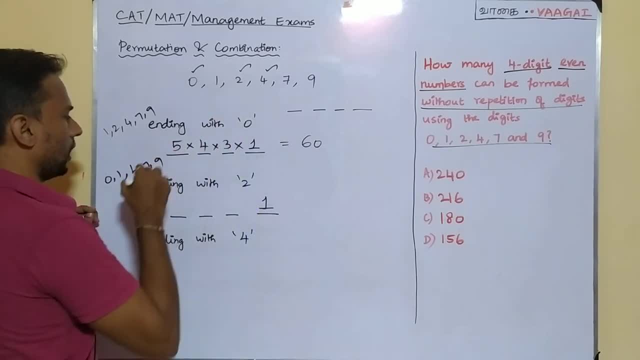 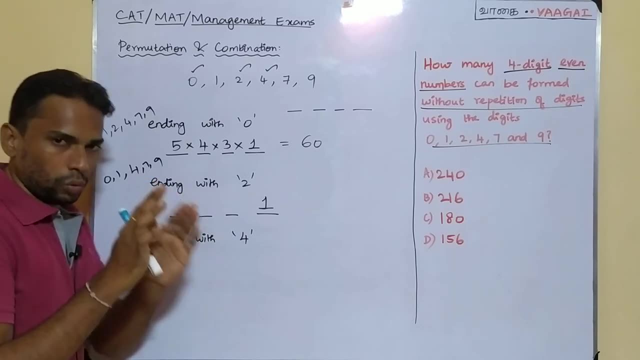 This 2 is already filled here. Now we have 4 or 7 or 9.. Okay, These are the other 5 digits left. The other 3 digits are to be filled with these 5 digits. only That we have to remember properly. 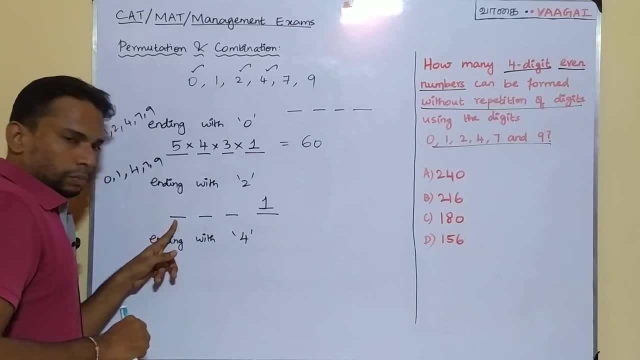 Okay, Alright, Yes, Fine, Now coming back again. start from the first slot. Okay, Now just see this slot. This slot can be filled in how many ways That we have to think Yes. Okay, Be clear. This slot can be filled in how many different ways We can fill this in, See here. 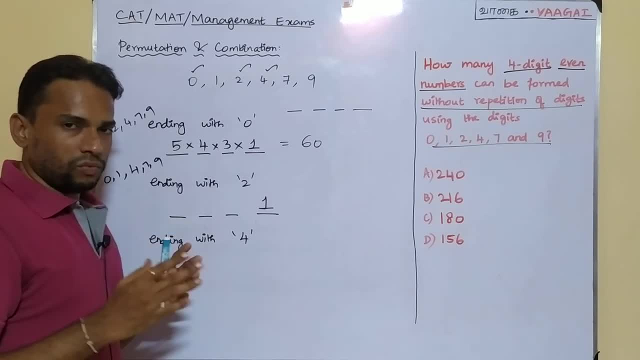 we have got 5 digits. Just hold on and think for a moment. Can you fill this slot with any one of these 5 digits? Is that possible? No, it is definitely not possible. Why? Because here, this time, we have the digits 0 also included. So in that case, in that case. 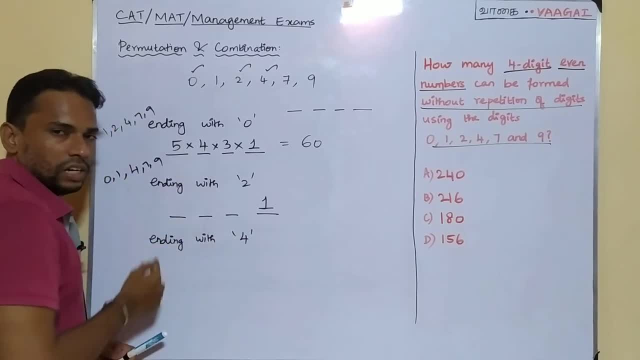 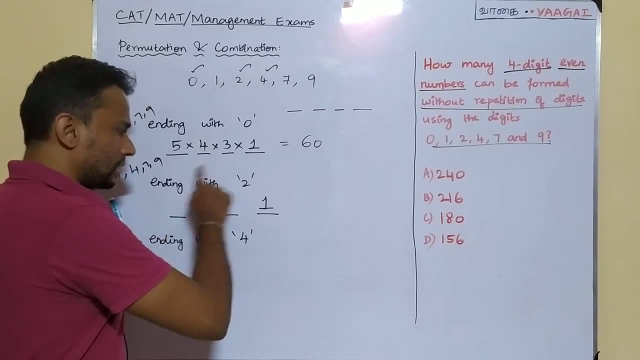 we cannot fill this first slot- I mean the first digit- with a 0. Why? Why we can fill this slot with a 0? Because the moment you fill this with a 0, this number will no more be a 4-digit number. 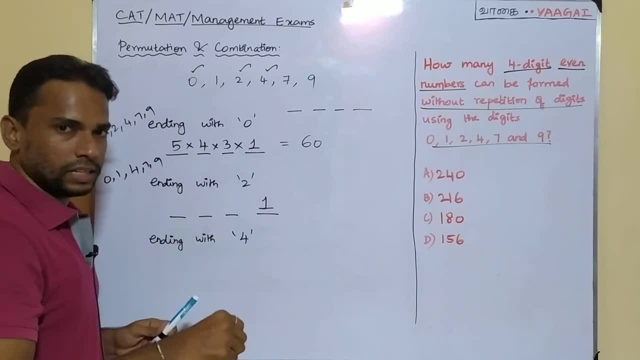 Is it or not? Why? Because you have a 4-digit number. So that means, in order to make this to be a 4-digit number, your first digit should be a non-0 digit. Is it clear? Yes, That is obvious. point right. I cannot have a 0 here. Why? Because if you fill, 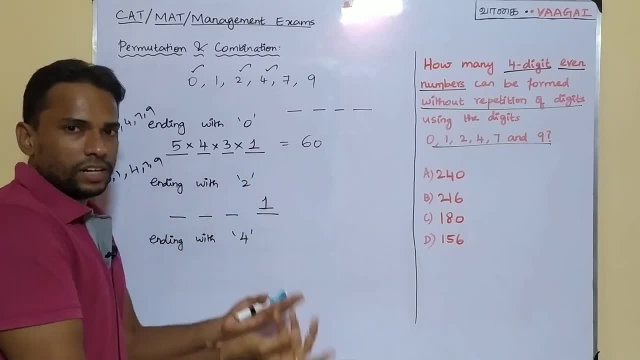 a 0 here. this will not become a 4-digit number, Maybe it will become a 3-digit number. It becomes a 3-digit number, Is it or not? So that means we should be cautious here in filling this first. 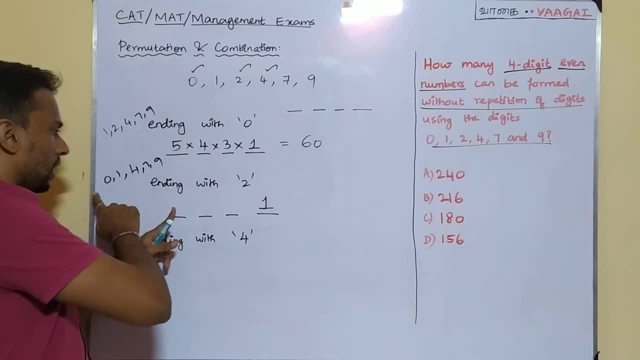 slot, And here you can fill any of these digits except this 0.. Okay, So in that case you will have how many ways in filling this first slot? You will have only 4 ways. Okay, Why? Because 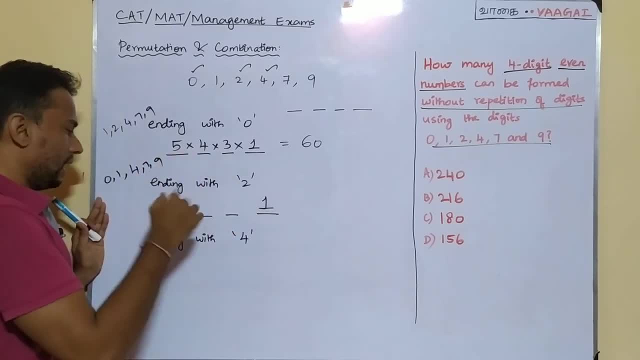 already 2 is filled. here We have got remaining 5 digits And now, except this 0, you have other 4 digits. Any one of those 4 can come here. So 4 ways to fill this first slot, Multiplied by 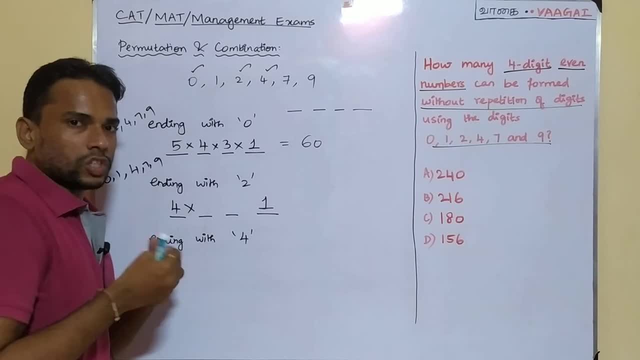 multiplied by. Now come to the second slot here. Now the second slot can be filled in how many different ways- That also we have to think here. Okay, How many ways it can be filled Now. now just think properly Now how we have filled. 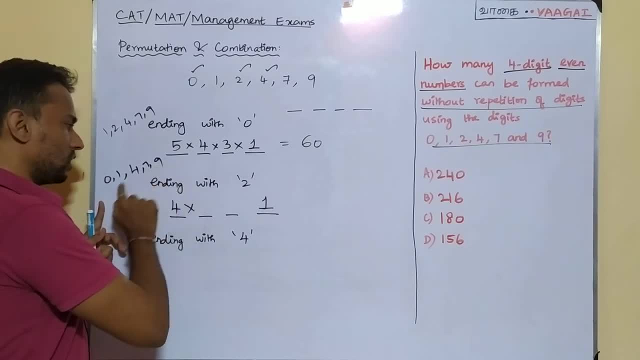 Out of these 5 remaining digits, one of these non-zero digits would have occupied this first slot. So now, what are the digits remaining? There are 3 non-zero digits available and 1: 0 is available. Now, again, we have got 4 remaining digits. Be clear, Okay, Be clear with this. We. 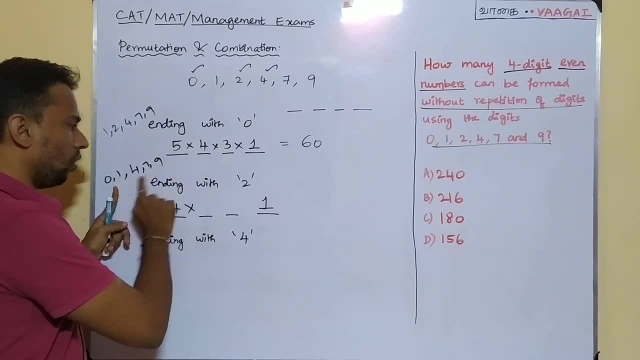 have other 3 non-zero digits because one of these 4 non-zero digits would have appeared here And for that reason there are only 3 non-zero digits and 1: 0. That means there are 4 digits available. Still, there are 4 digits available. Now any one of those 4 can come here. I mean this time. 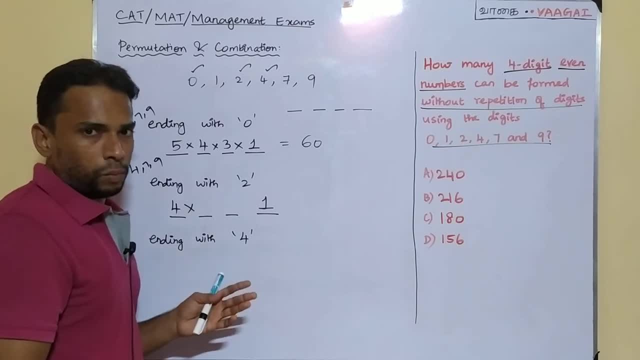 it will include that 0 also, Because this time, hereafter, there is no problem. When you take 0 here or here, it won't affect your questions condition. Why? Because when you have a 4-digit number, that in between digits can be 0. That will not affect your number. The thing is only the. 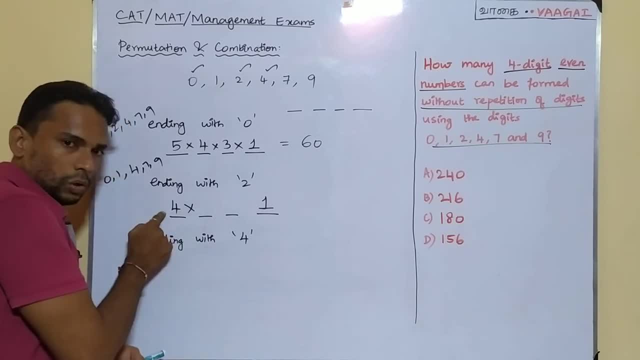 first digit can't be 0. That's the reason we restricted 0 to come here, But hereafter there is no problem. When you come here, you still have 3 non-zero digits and 1: 0, making there are 4. 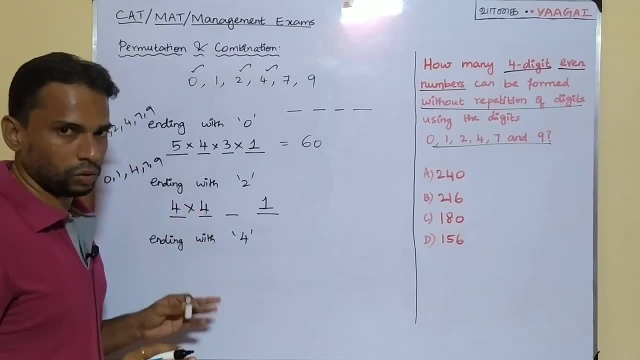 choices to fill this second slot. I hope it is clear to you now. Fine, Okay, Yes, Multiplied by Now coming here Now, how many slots will be there? I mean, how many ways to fill This one? 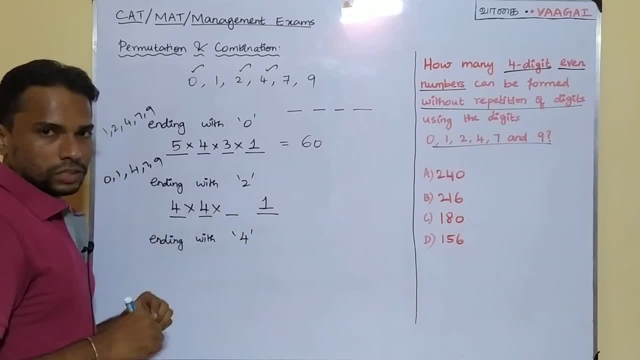 will be there To fill this you will have. what are the other things remaining? You have other 3 digits remaining, Okay, Because out of those 4, one of them will be filled and you will still have 3 more digits available. So 3 ways Okay. So now you multiply everything, So you will have. 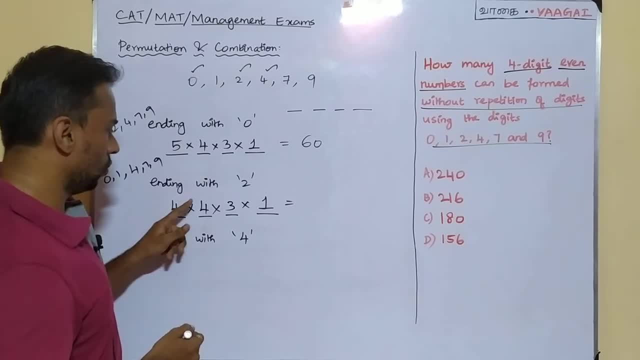 this will give you the possibility. So what will be? 4 into 4 into 3 into 1.. So this will be actually 48. Is it or not? So this will be 48. And yes, coming to the last case, What will be? 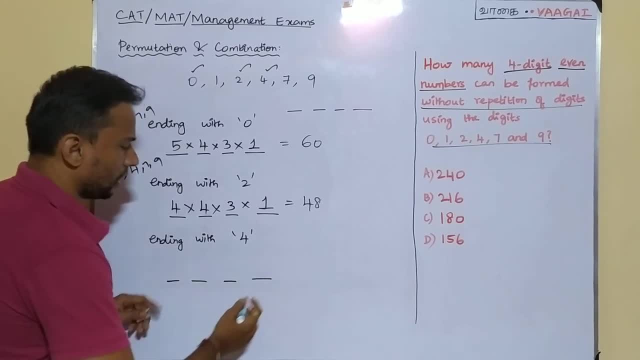 the last case. Last case: 1,, 2,, 3, 4.. Again, this one says this case. here we have our 4-digit number ending with the digit 4.. Okay, So that means here we are going to fill again one possible. 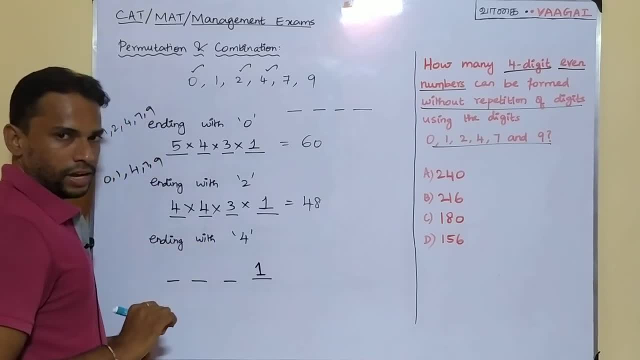 way. Okay, Again, this is going to be filled with one possible way, one possible way. So this is one possible way, And that one possibility is: what is this? digit 4.. Okay, All right. Yes, And now, when you fill this digit with 4, what will be the other digits remaining? You will have the. 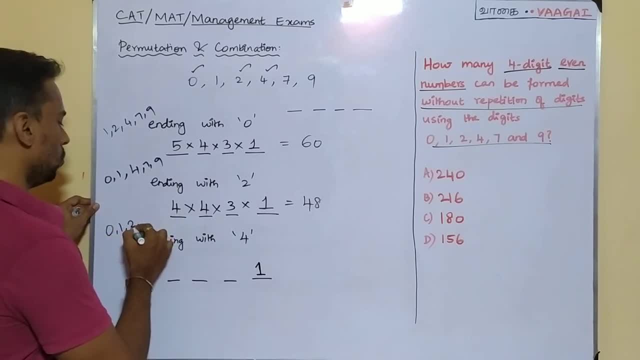 other digits to be 0,, 1,, 2, and then 7, and then 9.. See Yes, Clear Why? Because here in the previous case we had a 2.. The 2 is filled here, And here we have 4 is filled here. That's the. 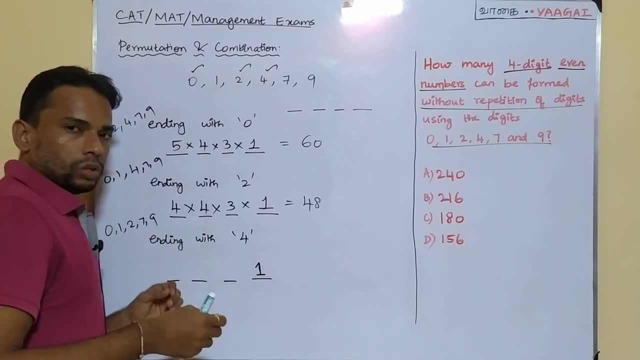 only change. Apart from that, the other conditions are going to be same. So that means, instead of the 4, we are going to have 4.. So that means, instead of the 4, we are going to have 4.. So 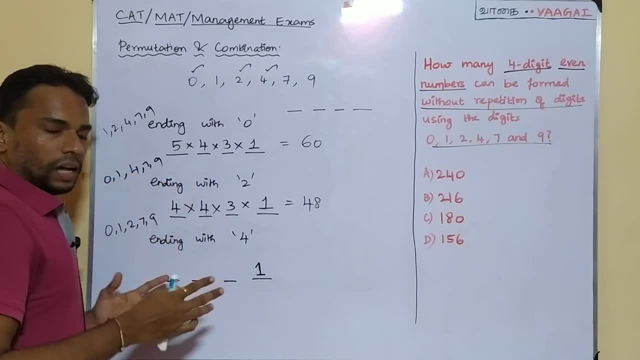 the remaining digits here. if you see, instead of 4, here we have 2.. But the others are going to be same only here, Is it, or not? Here again, if you come to fill the first 3 slots, it is again. 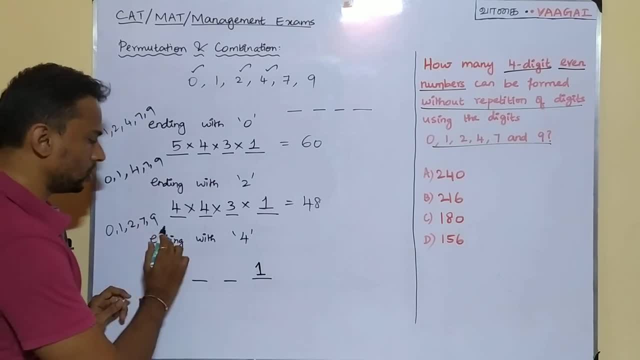 going to be the same. Why? Because you have, you have what You have: 4 non-0 digits and 1: 0., And that means this one can be filled with only 4 non-0 digits, Any one of these 4 non-0 digits. 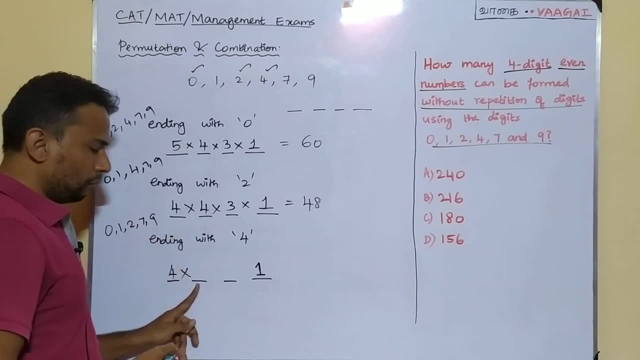 only So. that means 4 ways into. Again, you will have what when you come to the second slot? Again, the same story happens. Okay, Again, the same situation will be continued. You will have 3 non-0 digits and 1: 0. So 4 ways. Again. you will have what When you come to the second slot. 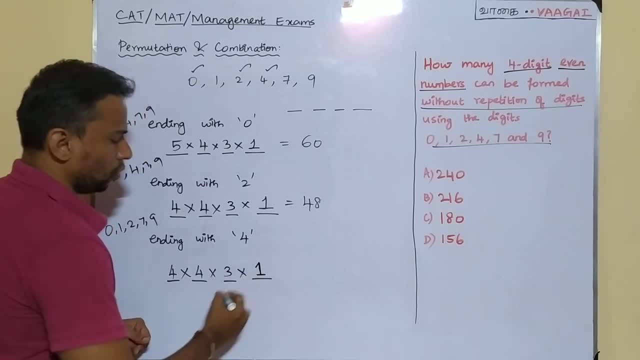 it is multiplied with again other 3 ways. Okay, So you will have 4 into 4 into 3 into 1.. Again, the product will be 48.. Okay, Yes, So this is where we should be very careful. Fine, Okay. 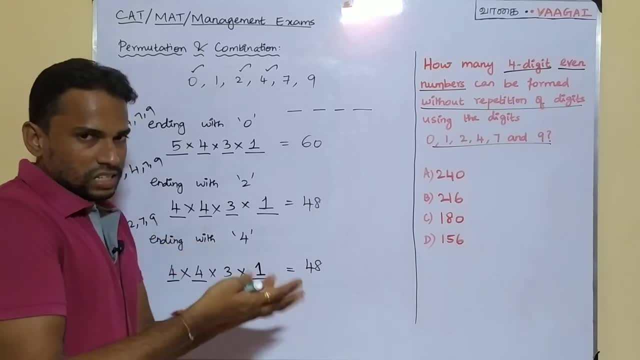 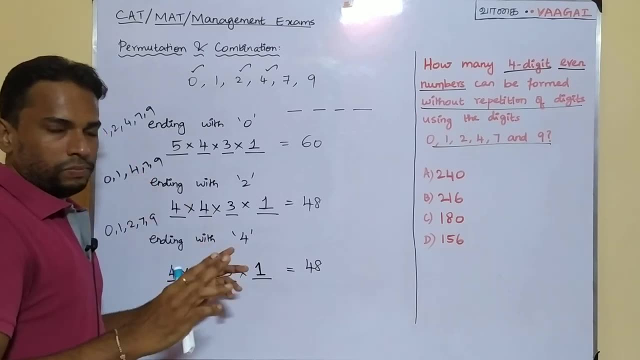 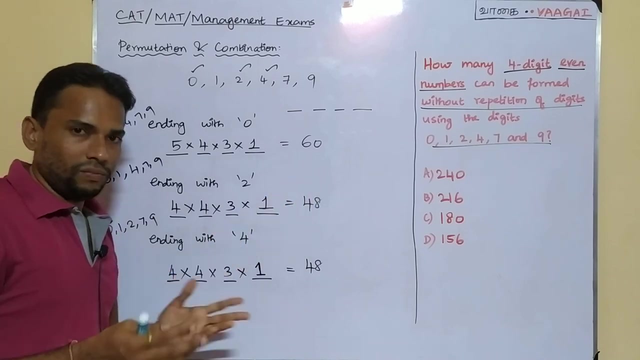 All right, And to make this problem even more comfortable, even more easy, what we can do is we can just combine these last 2 cases together. Okay, So we can just have this problem with just 2 cases. First case is ending with 0 and second case is ending with either 2 or 4.. That way also. 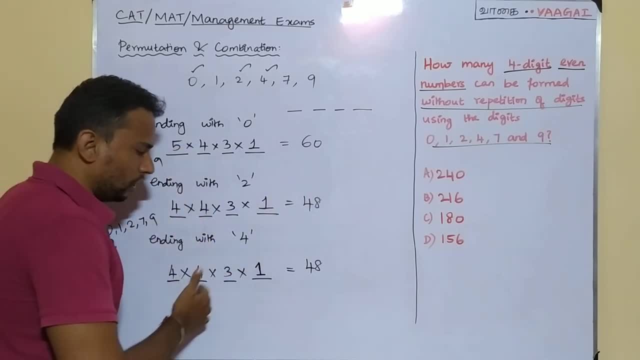 we can find out the difference, So we can just combine these last 2 cases together. Okay, So we can collide these 2.. Okay, So what happens is we will have 4 into 4, into 3, into 2 ways We can. 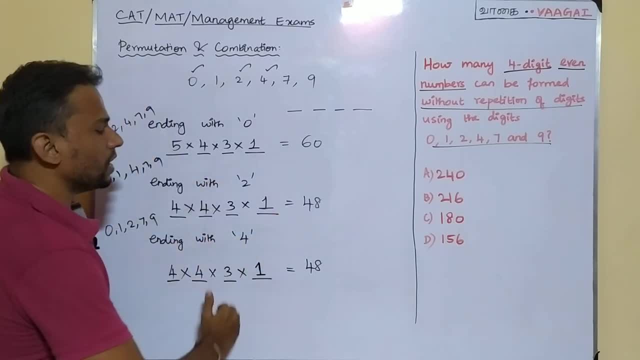 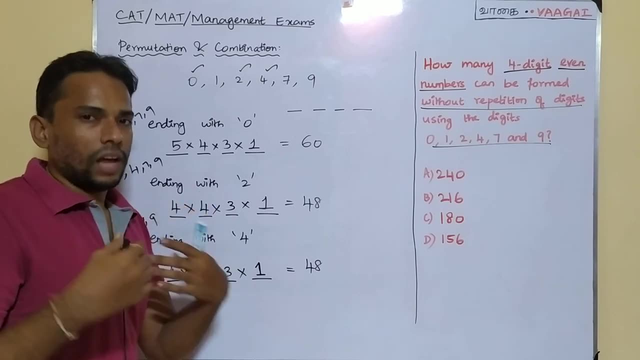 just combine those 2 conditions with 4 into 4, into 3, into 2 ways. Directly we can put that, But in order to make you give you understand, Okay, To give you the clarity, I just made it as: 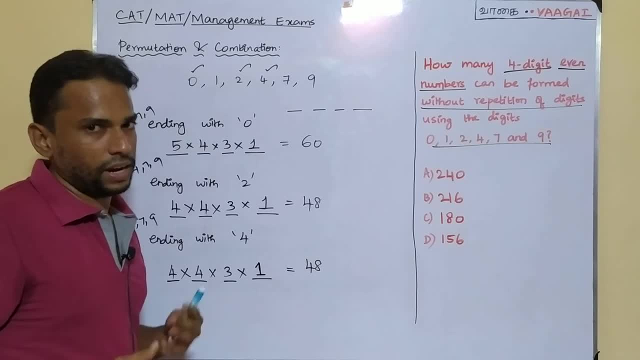 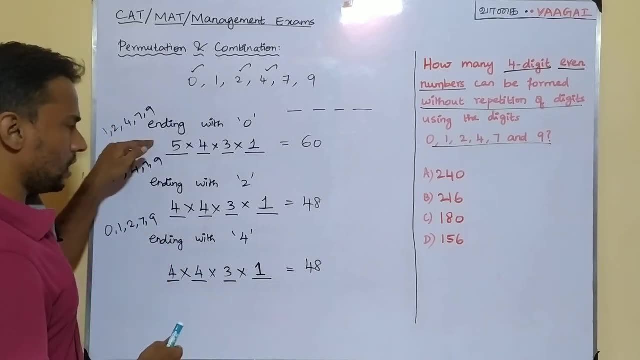 separate cases And later, after telling this, if I reveal, you may have some idea. That is the reason. Okay, Fine, Yes, So yeah, This is what we should be very careful here in working out this question. Okay, So see here. Here we have ending with 0.. 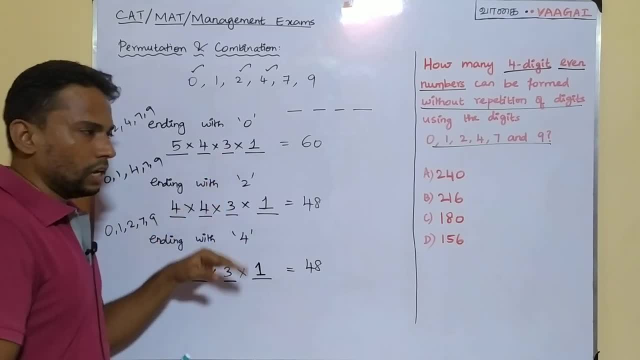 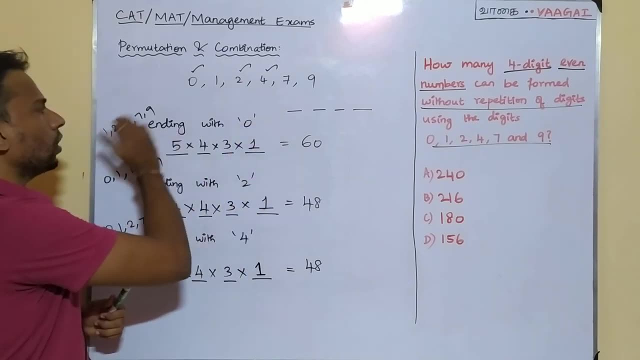 And here with ending with non-0, even digit, Okay. So those 2 cases are different And try to understand the difference. how we have Okay, So here, when you have the 0, all are non-0 digits. So that is why we have no restrictions here to fill the other 3 digits, We just directly. 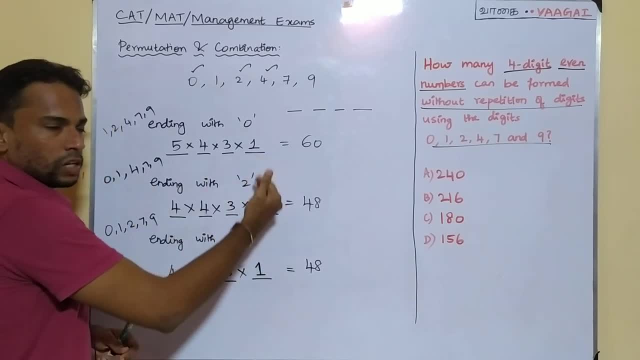 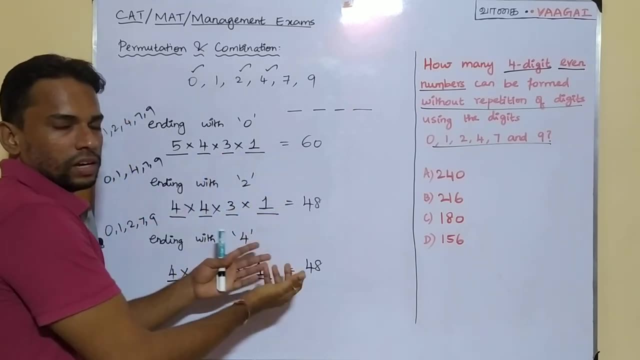 filled it. But when it comes to a non-0 digits here, Okay, So here we had 0. 0, and so we had this comfortability. But here, when it comes here, here we have to follow the restrictions, because this first digit is 0. So here we have 0. So here we have 0. So here we have 0. So. 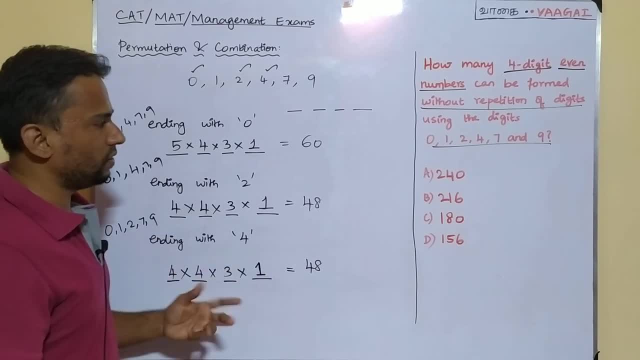 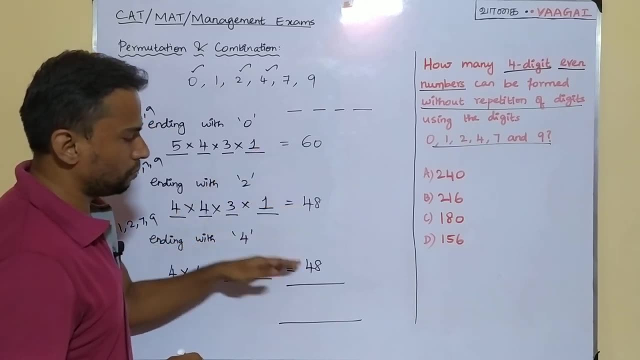 it cannot be 0.. That is the reason. Okay, Fine, Yes, So we have this. So, anyways, when you try to add everything, you will be getting the overall answer. Okay, So what is 60 plus 48 plus 48.. So